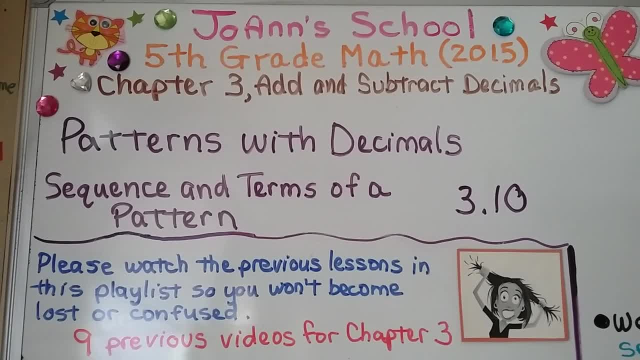 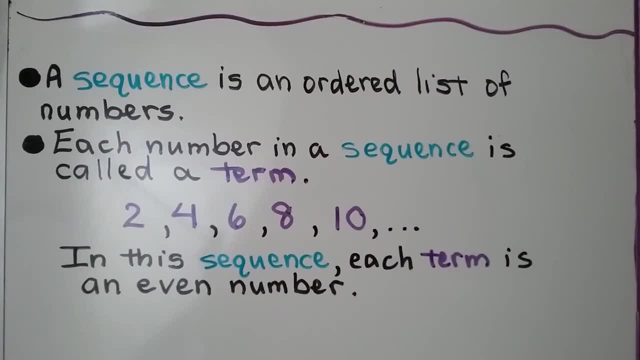 Lesson 3.10: Patterns with Decimals: Sequence and Terms of a Pattern. A sequence is an ordered list of numbers. Each number in a sequence is called a term. In this sequence, each term is an even number. We have 2,, 4,, 6, 8, 10.. They're all even numbers. We can use addition or subtraction to. 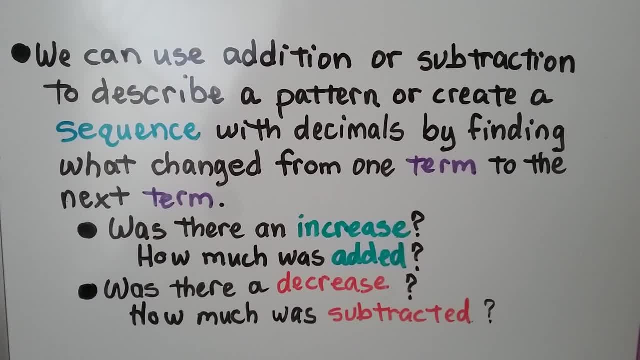 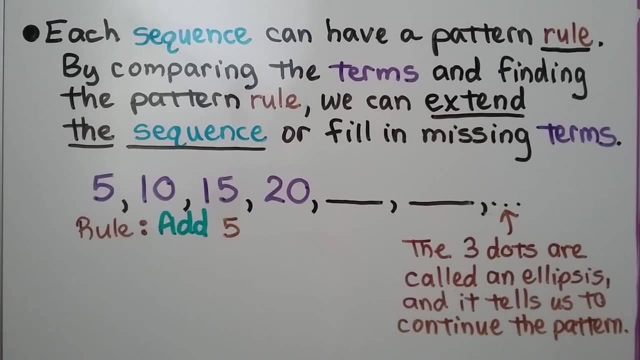 describe a pattern or create a sequence with decimals by finding what changed from one term to the next term. Was there an increase, How much was added, Was there a decrease? How much was subtracted? Each sequence can have a pattern rule By comparing the terms and finding the pattern. 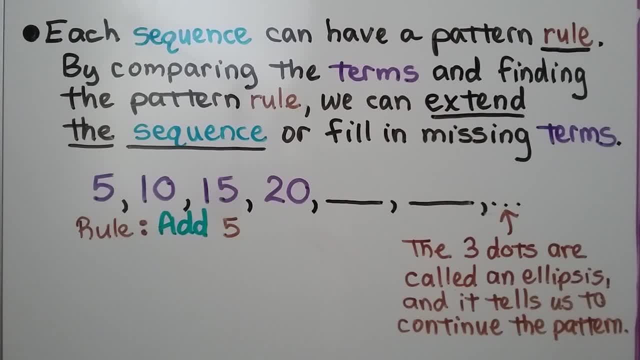 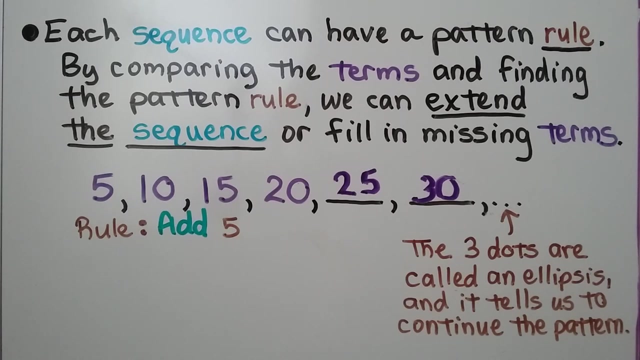 rule. we can extend the sequence or fill in missing terms. In this sequence we see the terms are 5, 10, 15, 20.. Then we have two missing ones. We can see the rule is: add 5.. We add 5,, we get 10.. We add 5,, we get 15.. We add 5,, we get 20.. And we can fill these in. If we add 5 to 20,, we get 25.. And if we add 5 more, we get 30.. You might see three little dots after a comma, After the last term. the three dots are called an ellipsis. 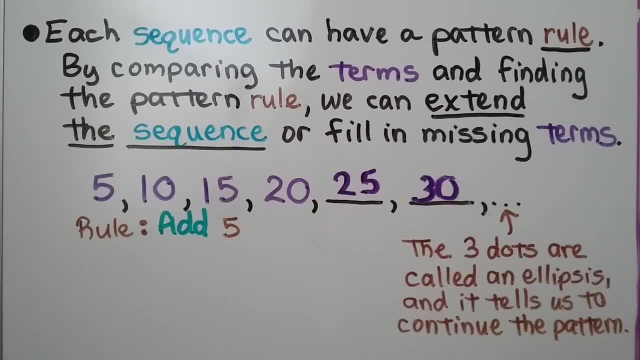 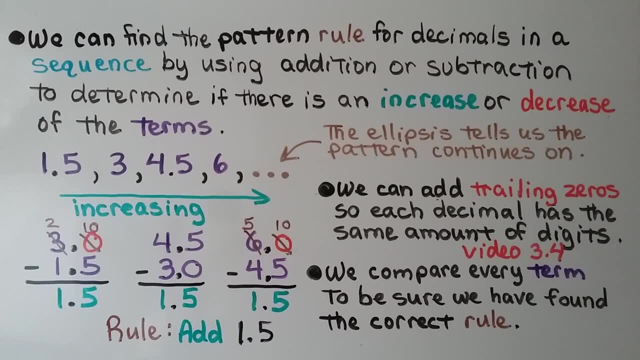 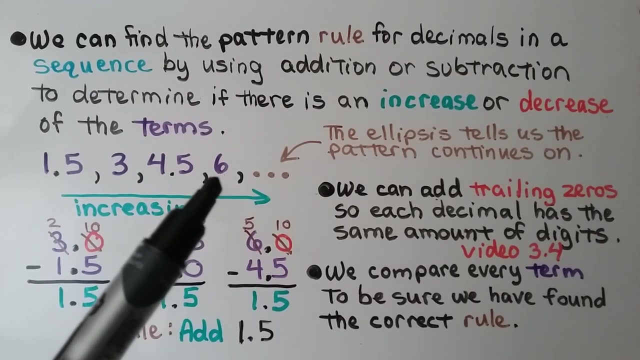 And it tells us to continue the pattern. We can find the pattern rule for decimals in a sequence by using addition or subtraction to determine is there an increase or decrease of the terms. We have 1 and 5 tenths, Then we have a 3. That's 3 whole. Then we have 4 and 5 tenths, Then we have a 6. That's a. 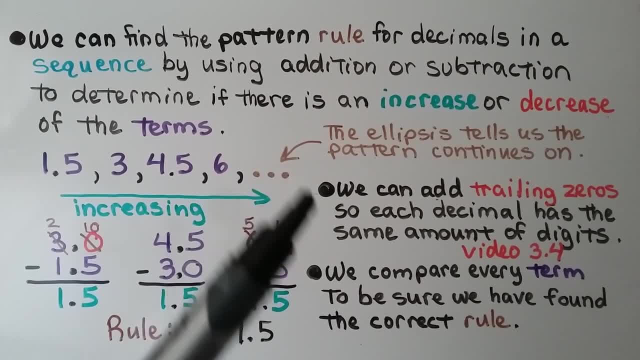 6 whole, And the ellipsis tells us that the pattern continues on. We can see that the that the terms are increasing. Each term is a little more than the one before it. We can add trailing zeros, so each decimal has the same amount of digits. 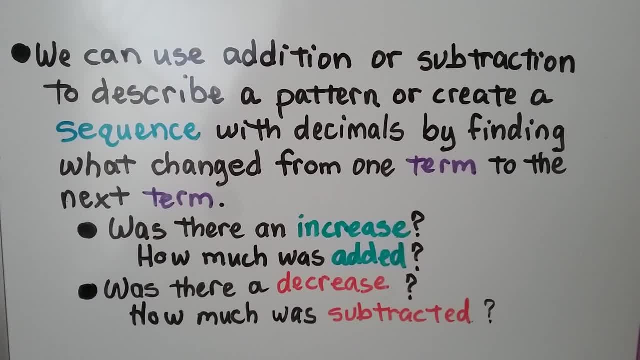 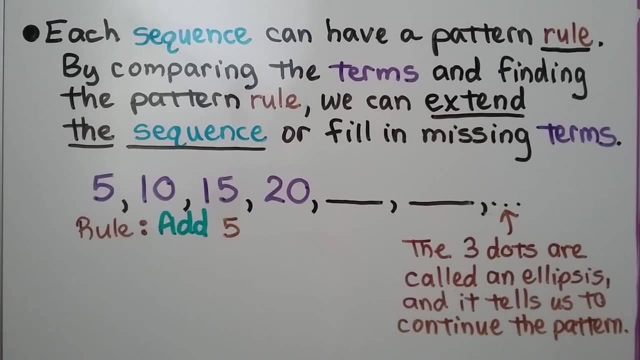 describe a pattern or create a sequence with decimals by finding what changed from one term to the next term. Was there an increase, How much was added, Was there a decrease? How much was subtracted? Each sequence can have a pattern rule By comparing the terms and finding the pattern. 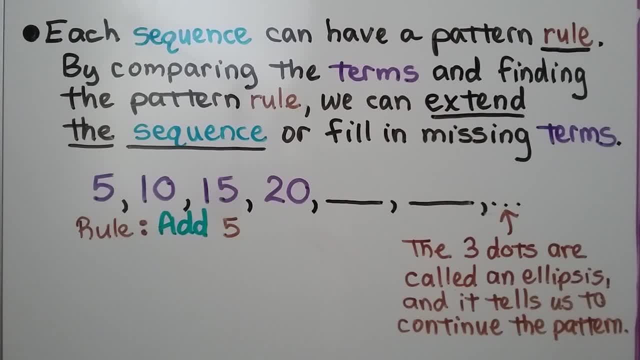 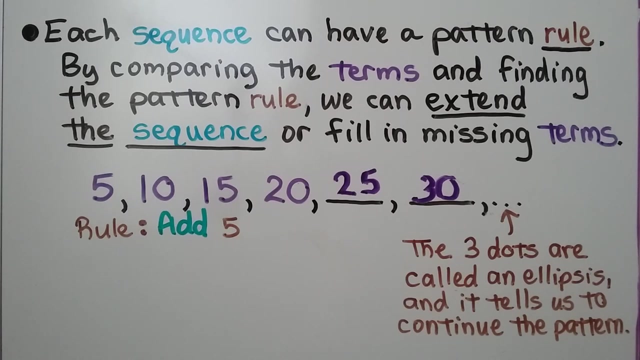 rule. we can extend the sequence or fill in missing terms. In this sequence we see the terms are 5, 10, 15, 20.. Then we have two missing ones. We can see the rule is: add 5.. We add 5,, we get 10.. We add 5,, we get 15.. We add 5,, we get 20.. And we can fill these in. If we add 5 to 20,, we get 25.. And if we add 5 more, we get 30.. You might see three little dots after a comma, After the last term. the three dots are called an ellipsis. 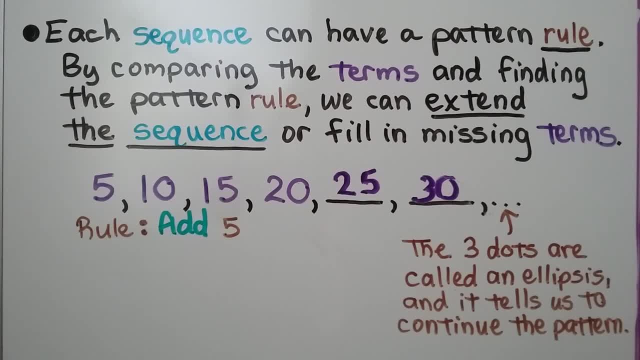 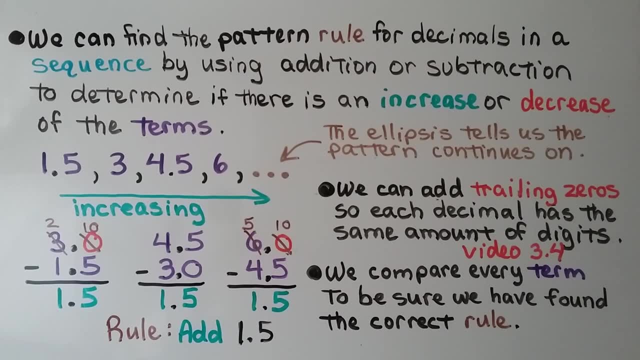 And it tells us to continue the pattern. We can find the pattern rule for decimals in a sequence by using addition or subtraction to determine is there an increase or decrease of the terms. We have 1 and 5 tenths, Then we have a. 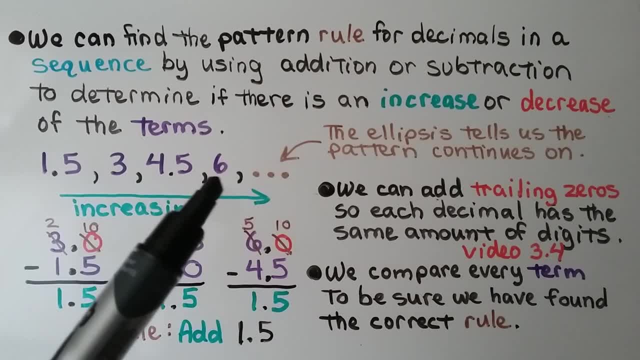 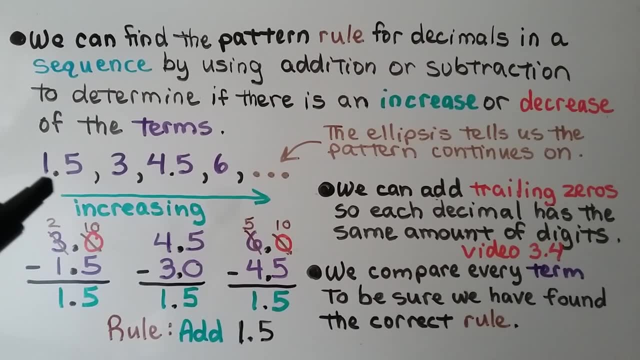 3. That's three whole, Then we have 4 and 5 tenths, Then we have a 6. That's a six whole, And the ellipsis tells us that the pattern continues on. We can see that the terms are increasing. 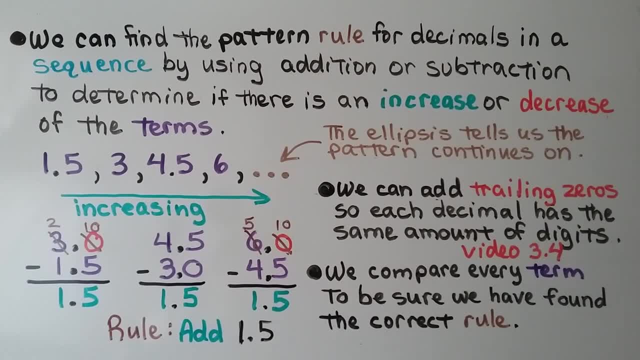 Each term is a little more than the one before it. We can add trailing zeros so each decimal has the same amount of digits. We learned about trailing zeros in video 3.4.. So if we have 3 and we want to find the difference between 3, 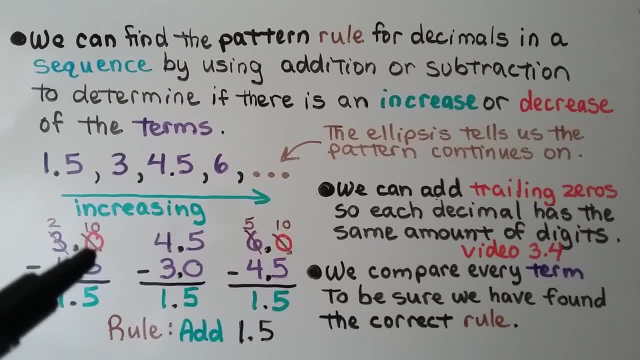 and 1 and 5 tenths. we're going to subtract to find the difference And we can add a trailing 0 and a decimal point to the right of the 3, so we can subtract And we see it's 1 and 5 tenths. 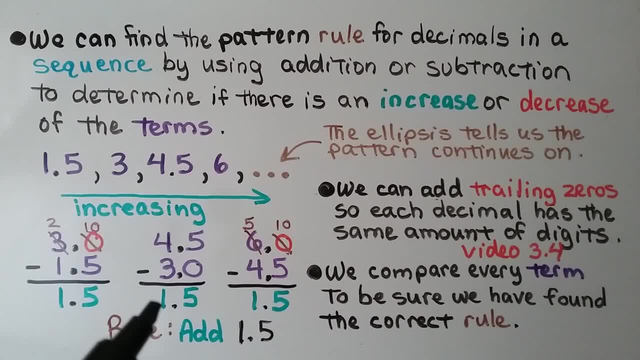 Now we find the difference between 4 and 5 tenths and 3. And we find it's 1 and 5 tenths again. Now we find the difference between 6 and 4 and 5 fifths. We see it's 1 and 5 tenths again. 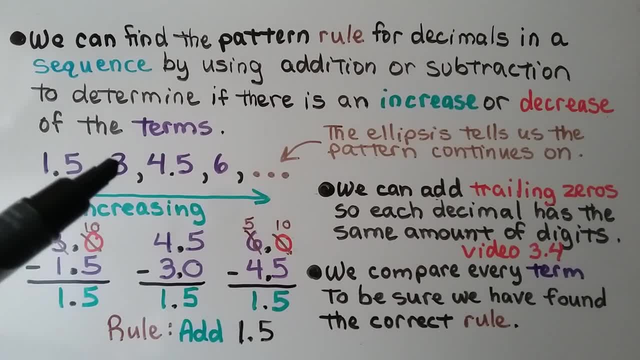 We learned about trailing zeros in video 3.4.. So if we have 3 and we want to find the difference between 3 and 1 and 5 tenths, we're going to subtract to find the difference And we can add a trailing 0 and a decimal point. 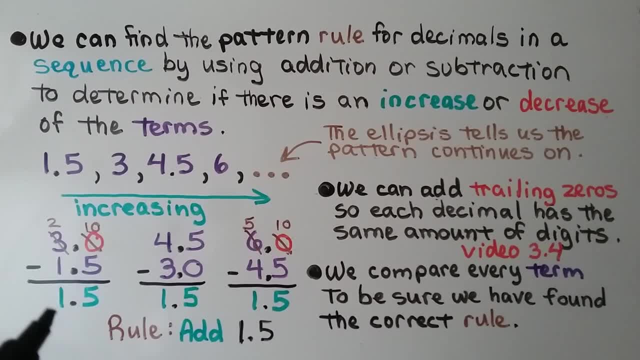 to the right of the 3, so we can subtract And we see it's 1 and 5 tenths. Now we find the difference between 4 and 5 tenths and 3. And we find it's 1 and 5 tenths again. 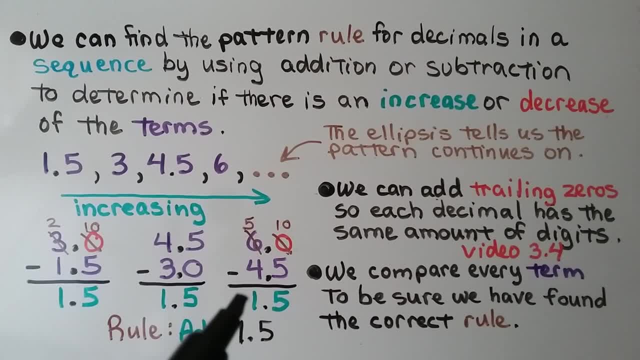 Now we find the difference between 6 and 4 and 5 fifths. We see it's 1 and 5 tenths. again, We compare every term to be sure we have found the correct rule, And the rule is to add 1 and 5 tenths. 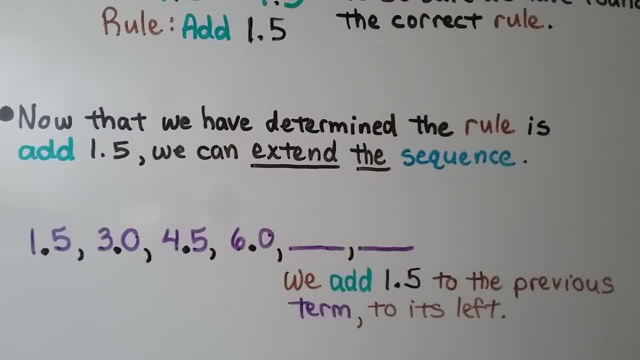 Now that we've determined the rule is add 1 and 5 tenths, we can extend this And the rule is to add 1 and 5 tenths to the previous term and add 1 and 5 tenths to the previous term in the sequence. 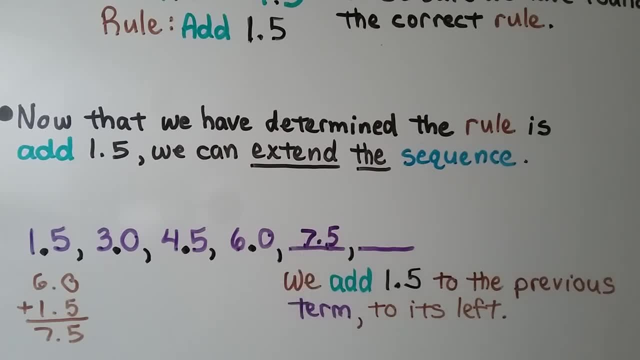 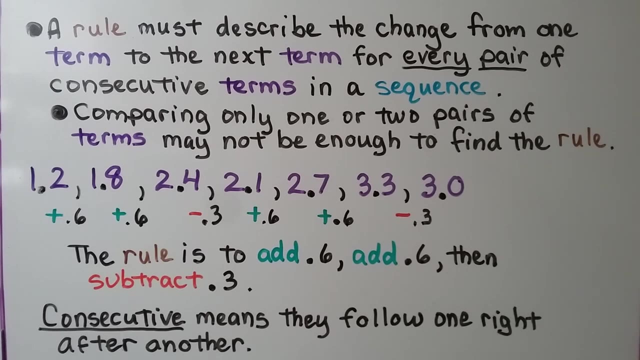 We have 6.. We're going to add 1 and 5 tenths. That's 7 and 5 tenths. Now we need to add another 1 and 5 tenths. We add 1 and 5 tenths to the previous term, to its left. 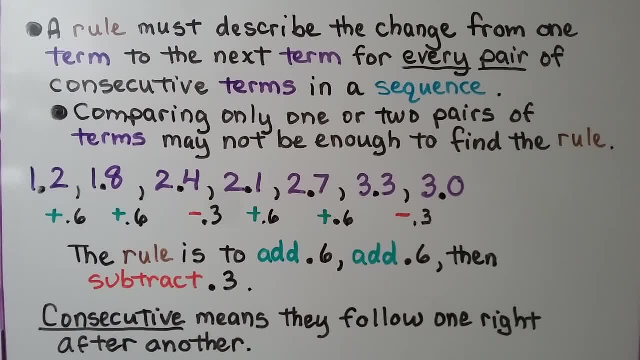 terms in a sequence. Comparing only one or two pairs of terms may not be enough to find the rule. We have 1 and 2 tenths, then it goes to 1 and 8 tenths. We added 6 tenths For the next term. it's 2 and 4 tenths. we added another 6 tenths. Now, if 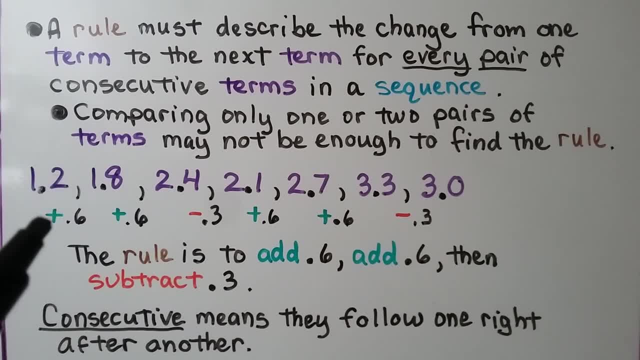 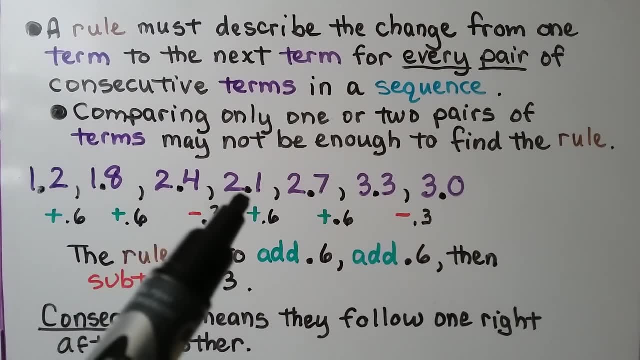 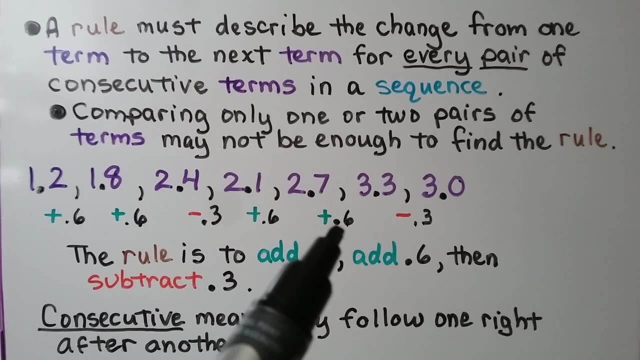 we had just stopped here, we would think that the rule is to add 6 tenths. but if we continue on we see that it goes down. We subtracted 3 tenths. Then we find the difference between these two terms and find that we add 6 tenths again. Then we add 6 tenths again. 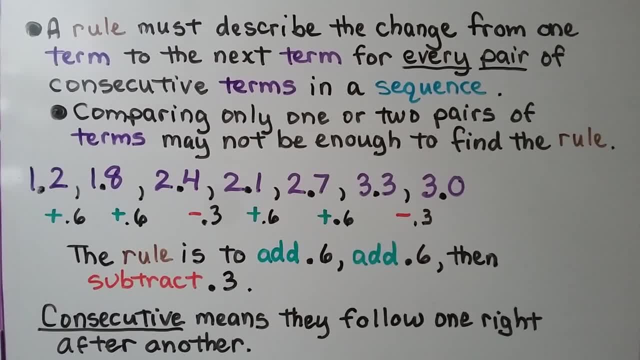 Then we subtract 3 tenths. So the rule is to add 6 tenths, then add 6 tenths, then subtract 3 tenths. We can have a rule that's got addition and subtraction in it. We can even have a. 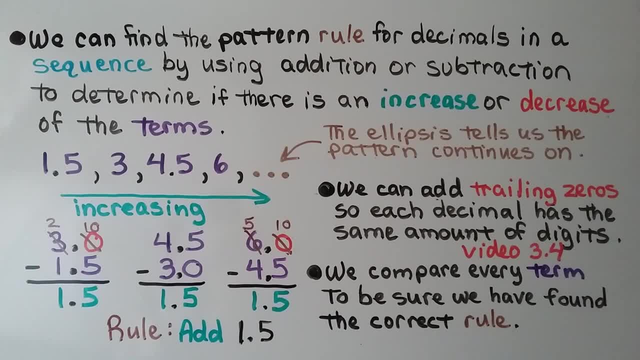 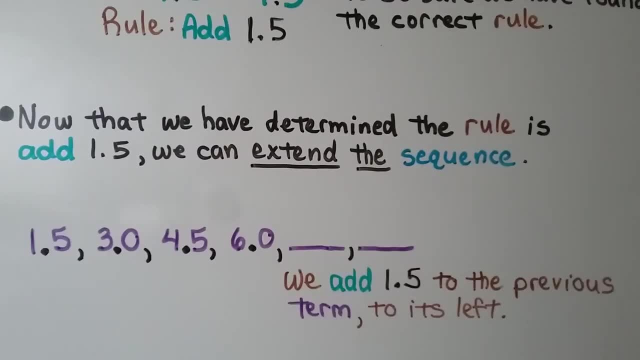 We compare every term to be sure we have found the correct rule, And the rule is to add 1 and 5 tenths. Now that we've determined the rule is add 1 and 5 tenths, we can extend this. Let's look at the sequence. 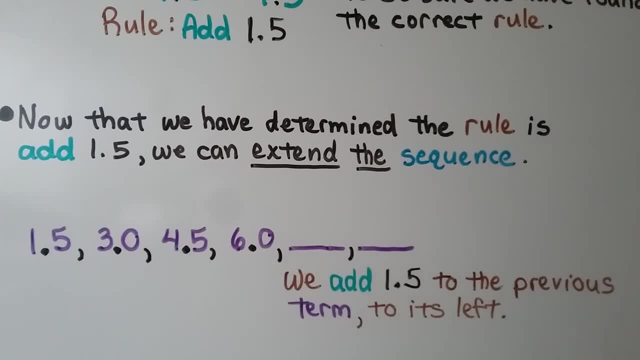 We have 6.. We're going to add 1 and 5 tenths. That's 7 and 5 tenths. Now we need to add another 1 and 5 tenths. We add 1 and 5 tenths to the previous term, to its left. 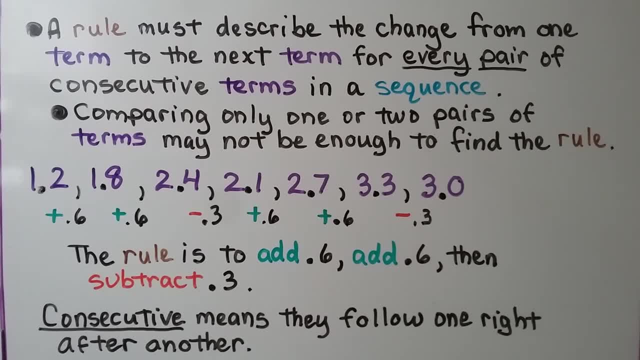 A rule must describe the change from one term to the next term for every pair of consecutive terms In a sequence. Comparing only one or two pairs of terms may not be enough to find the rule. We have 1 and 2 tenths. 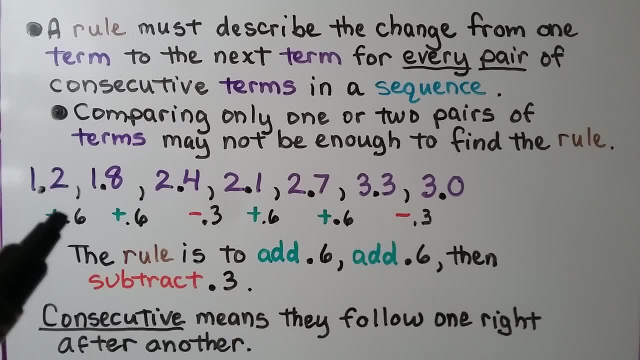 Then it goes to 1 and 8 tenths. We added 6 tenths. For the next term it's 2 and 4 tenths. We added another 6 tenths. Now, if we had just stopped here, we. 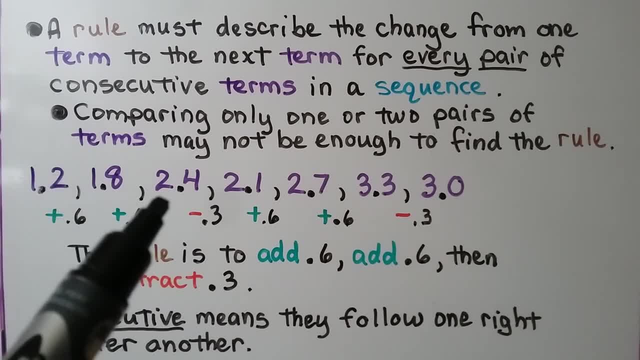 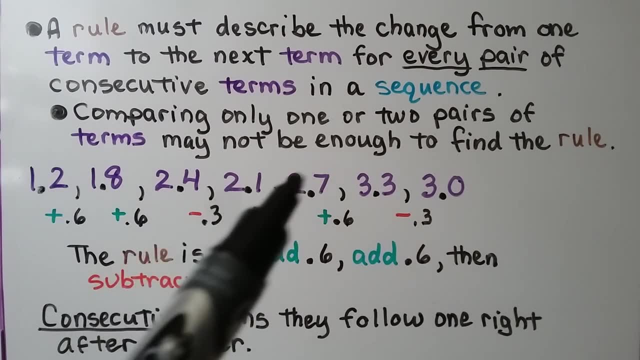 would think that the rule is to add 6 tenths, But if we continue on we see that it goes down. We subtracted 3 tenths, Then we find the difference between these two terms and find that we add 6 tenths again. 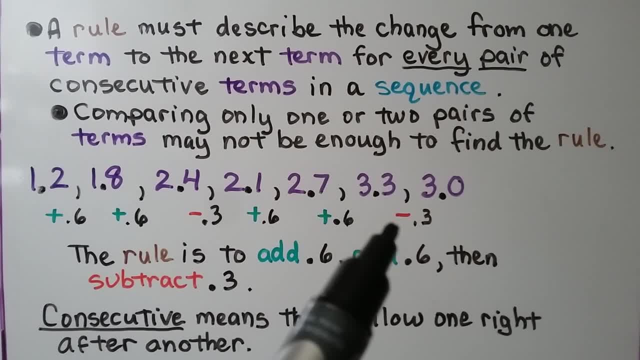 Then we add 6 tenths again, Then we subtract 3 tenths. So the rule is to add 6 tenths, Then add 6 tenths, Then subtract 3 tenths. We can have a rule that's got addition and subtraction in it. 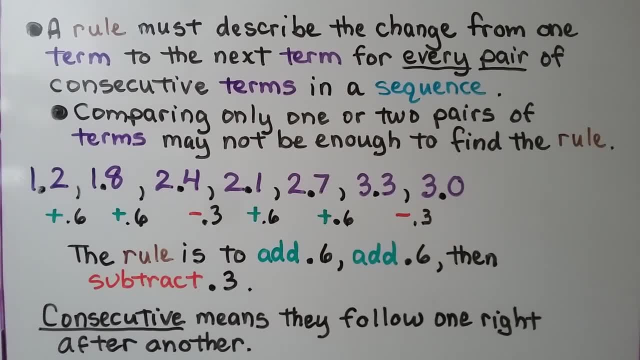 We can even have a rule that's got division and multiplication in it. And consecutive means they follow 1 right after any member of the binary vec who had에요 будущ MH10. And consecutive means they follow 1 right after any member of the binary vec who had Rhodesっと. 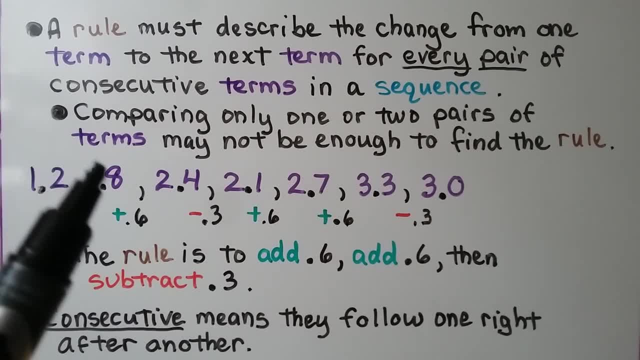 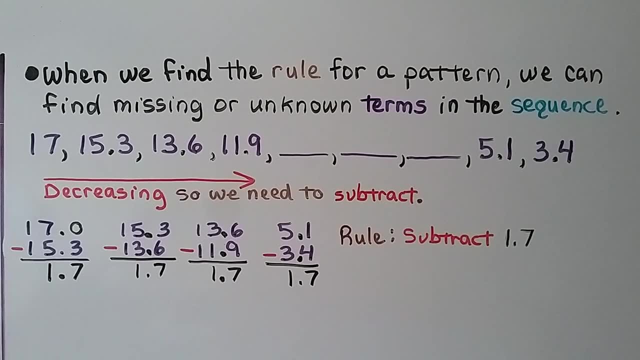 another. so consecutive terms are the terms in order, one after another. When we find the rule for a pattern we can find missing or unknown terms in the sequence. So here we've got missing terms in the middle. We see it goes from 17 to 15 and 3 tenths down to 13 and 6 tenths down to 11 and 9 tenths. 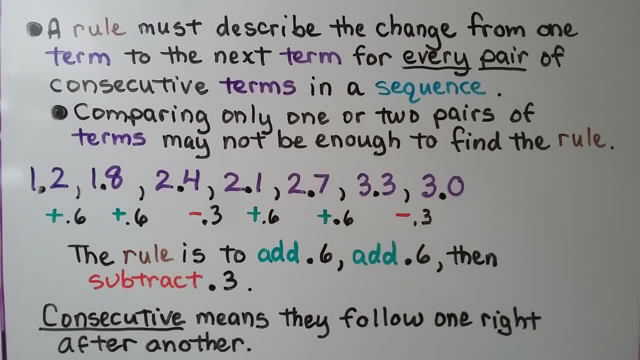 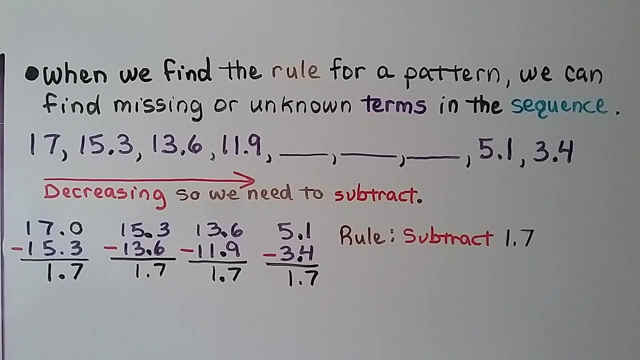 rule that's got division and multiplication in it And consecutive means they follow one right after another. So consecutive terms are the terms in order, one after another. When we find the rule for a pattern we can find missing or unknown terms in the sequence. So here we've got missing terms in the middle. We 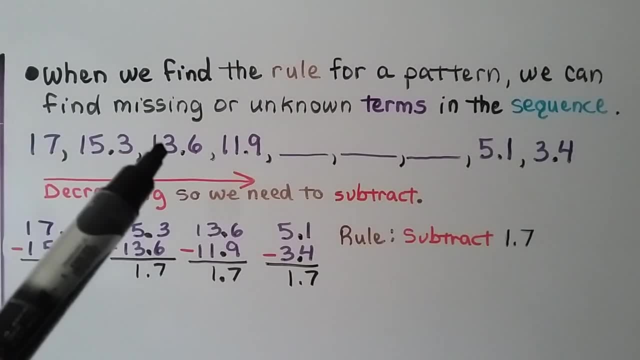 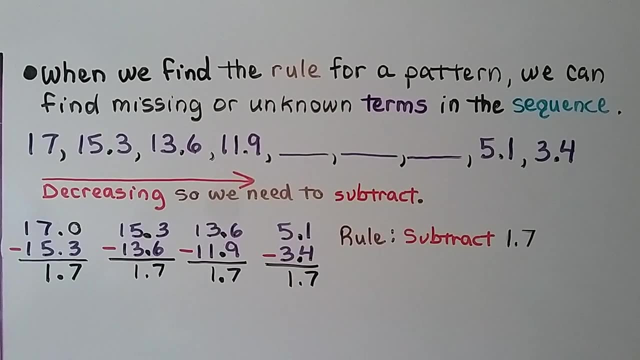 see, it goes from 17 to 15 and 3 tenths, down to 13 and 6 tenths and then it goes down to 11 and 9 tenths. So they're decreasing. So we know we need to subtract. We start with. 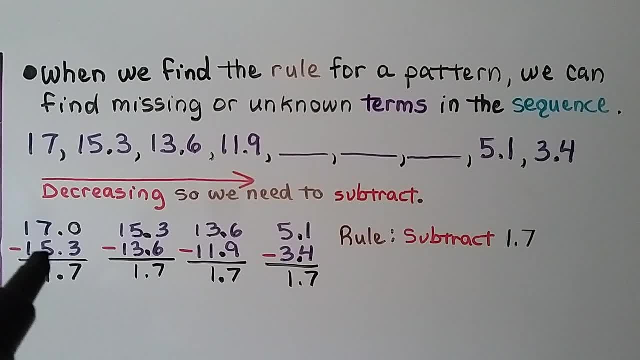 17. We can put a trailing zero here, so we can subtract 15 and 3 tenths And we get 1 and 7 tenths. 1 and 7 tenths was subtracted to get to 15 and 3 tenths And to get to 13. 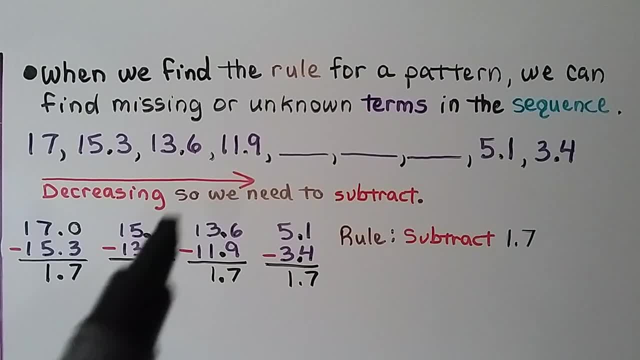 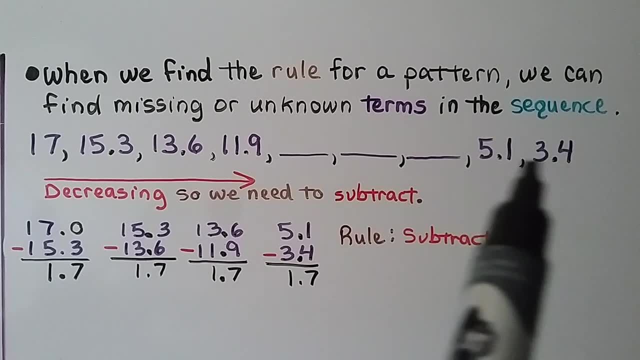 and 6 tenths. another 1 and 7 tenths was subtracted To get to 11 and 9 tenths. another 1 and 7 tenths was subtracted. And we check, We check between here and see the difference is 1 and 7 tenths. That means we need to subtract. 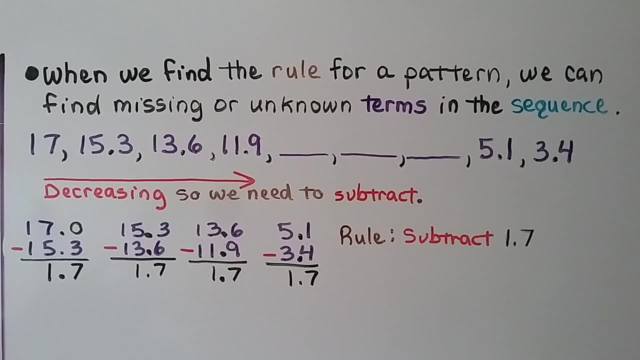 1 and 7 tenths. to find each of those terms, We subtract 1 and 7 tenths from 11 and 9 tenths and we get 10 and 2 tenths. We subtract another 1 and 7 tenths and get 8 and 5 tenths. We subtract. 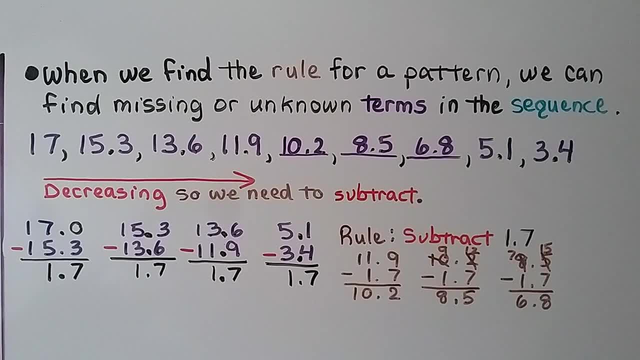 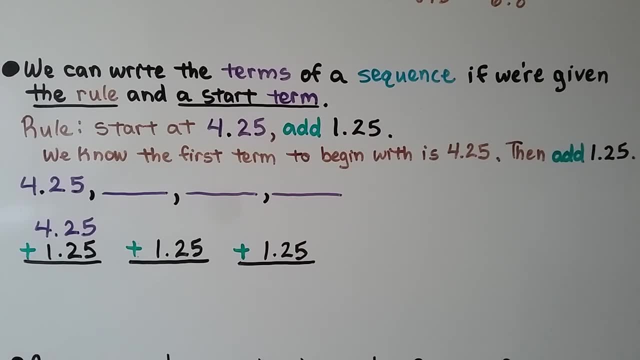 another 1 and 7 tenths and get 6 and 8 tenths. We can write the terms of a sequence if we're given the rule and a start term. It says the rule: we start at 4 and 25 hundredths and. 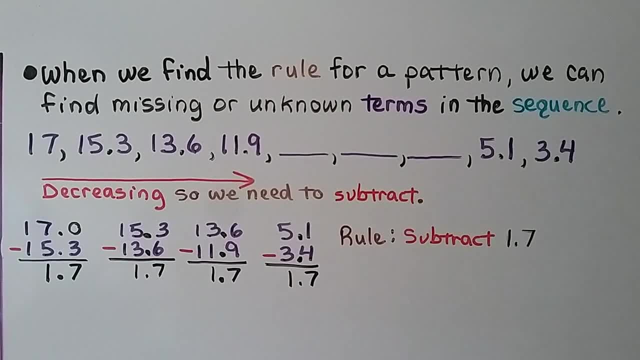 so they're decreasing. So we know we need to subtract. We start with 17,. we can put a trailing zero here. so we can subtract 15 and 3 tenths and we get 1 and 7 tenths. One and seven tenths was subtracted to get to 15 and 3 tenths. 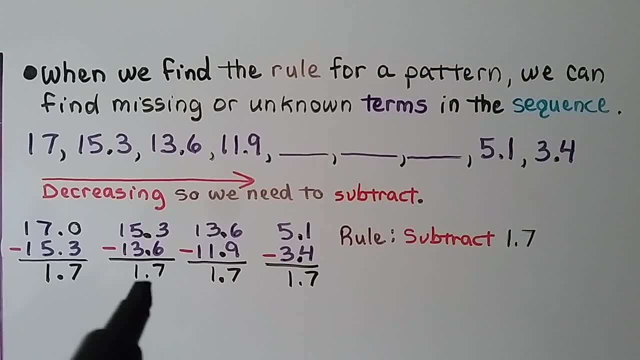 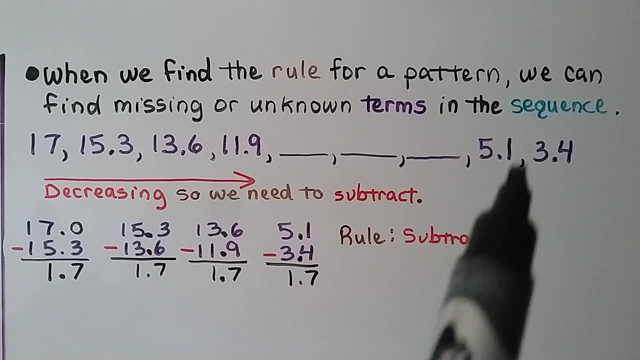 And to get to 13 and 6 tenths, another one and seven tenths was subtracted. To get to 11 and 9 tenths, another one and seven tenths was subtracted. And we check between here and see the difference is one and seven tenths. 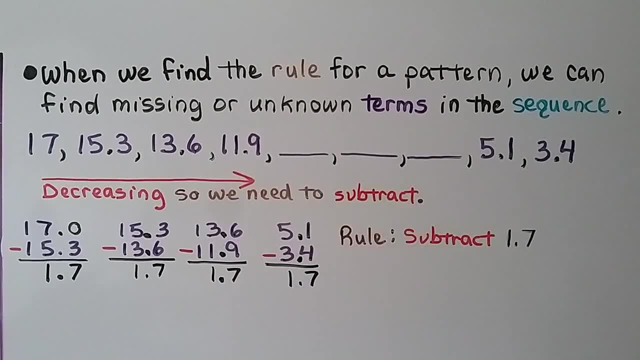 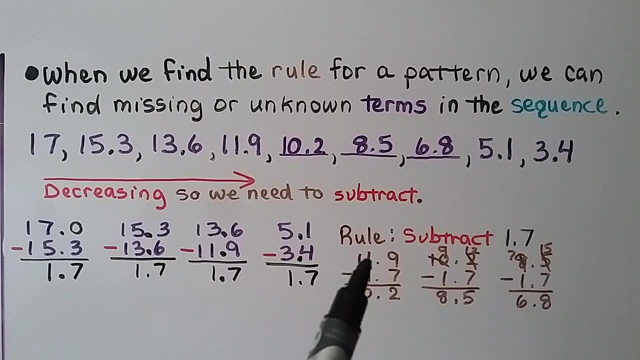 That means we need to subtract one and seven tenths to find each of those terms. We subtract one and seven tenths from 11 and 9 tenths and we get 10 and 2 tenths. We subtract another one and seven tenths and get 8 and 5 tenths. 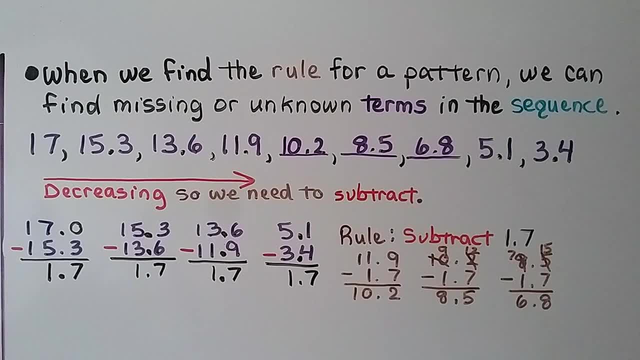 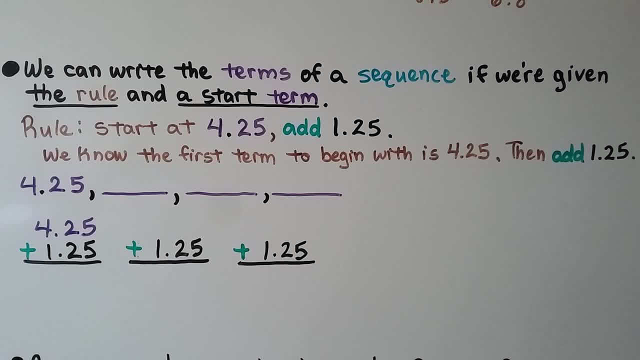 We can write the terms of a sequence if we're given the rule. if we're given the rule and a start term, It says the rule: we start at 4 and 25 hundredths and add 1 and 25 hundredths. 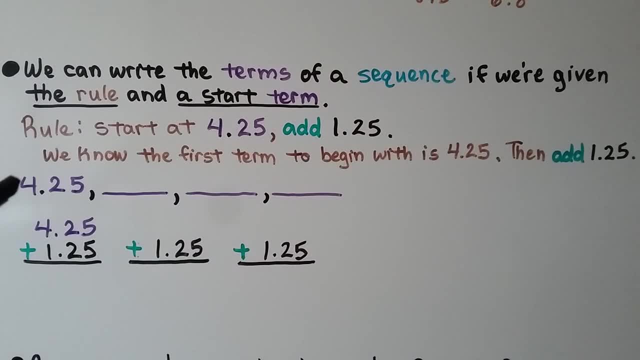 So we know the first term to begin with is 4 and 25 hundredths, It told us. start at 4 and 25 hundredths, Then we add 1 and 25 hundredths to get the next term. It's 5 and 50 hundredths. 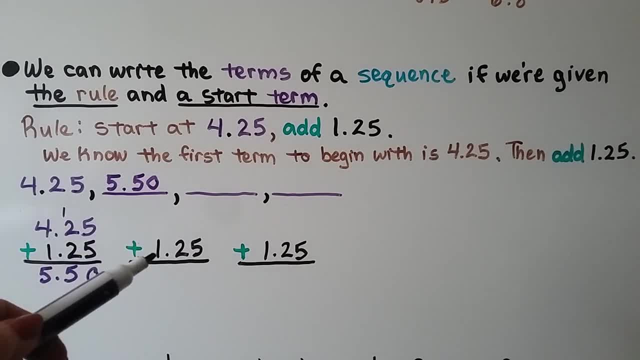 Now we can add 5 and 50 hundredths to 1 and 25 hundredths to get the next term. We get 6 and 75 hundredths. Now we can add 1 and 25 hundredths to this term to get the last one. 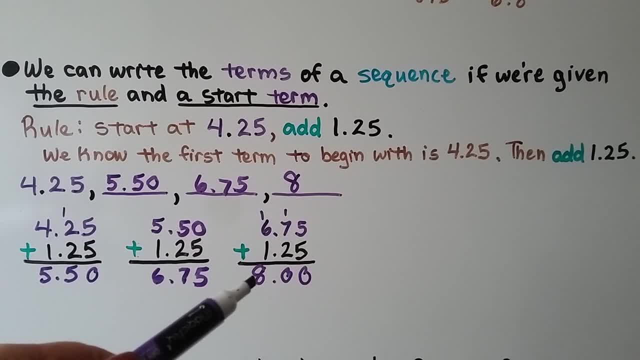 And we can remove the trailing zeros. We had 8 ones. That's just 8 whole, with no tenths and no hundredths, So we can just write an 8. We can even write this As 5 and 5 tenths if we wanted to. 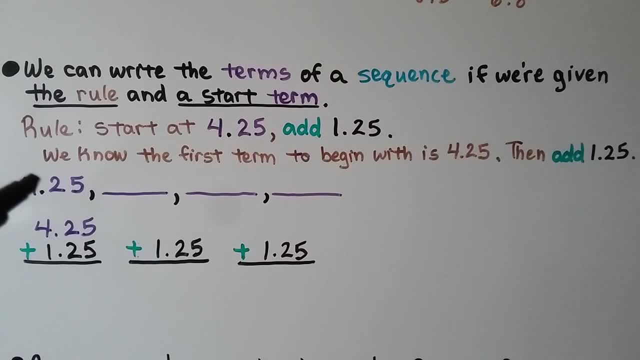 add 1 and 25 hundredths. So we know the first term to begin with is 4 and 25 hundredths, It told us. start at 4 and 25 hundredths, Then we add 1 and 25 hundredths to get the next term. 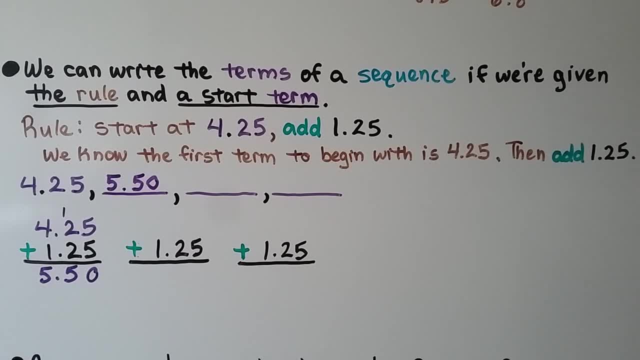 It's 5 and 50 hundredths Now we can add 5 and 50 hundredths to 1 and 25 hundredths to get the next term. We get 6 and 75 hundredths. Now we can add 1 and 25 hundredths to this term to get the last one. 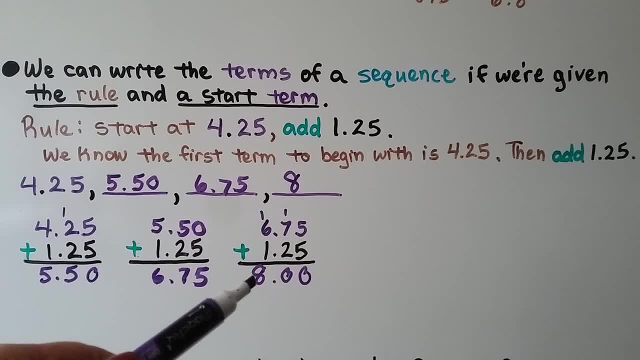 And we can remove the trailing zeros. We had 8 ones. That's just 8 whole, with no tenths and no hundredths, So we can just write an 8. We can even write this as 5 and 5 tenths if we wanted to. 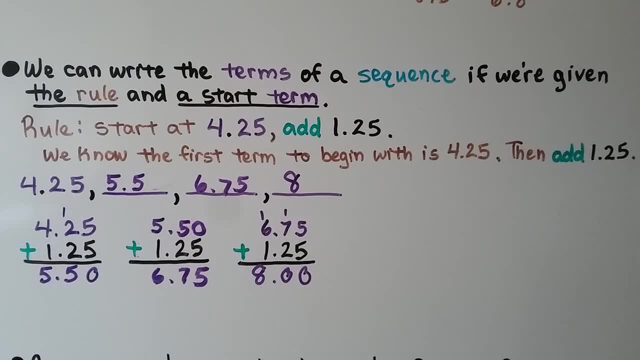 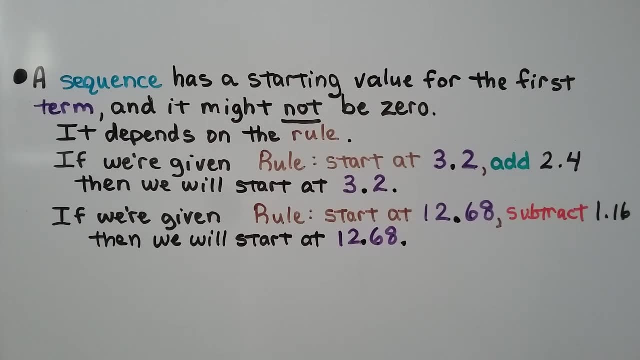 We can remove that trailing zero. A sequence has a starting value for the first term and it might not be zero. It depends on the rule. If we're given that the rule says: start at 3 and 2 tenths and add 2 and 4 tenths, 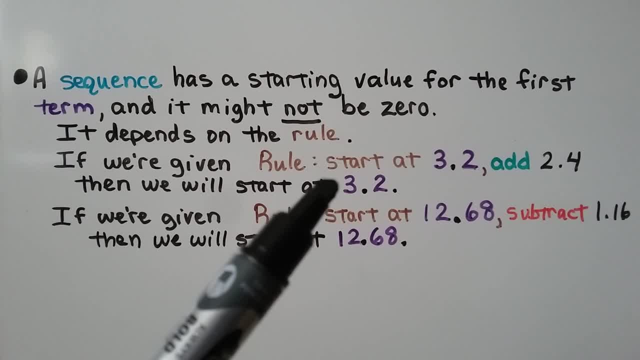 then our first term will be 3 and 2 tenths. That's where we'll start. Then we'll add 2 and 4 tenths to it to get the next term. Add another 2 and 4 tenths And, if we're given the rule, start at 12 and 68 hundredths and subtract 1 and 16 hundredths. 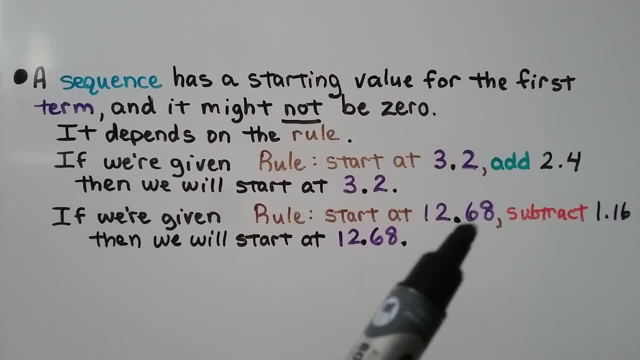 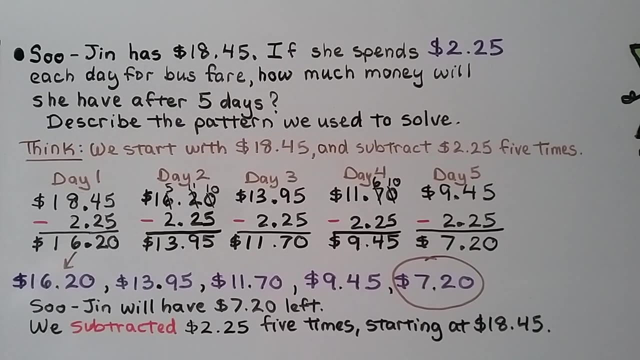 then we're going to start at 12 and 68 hundredths. That will be our first term. Then we'll subtract 1 and 16 hundredths from it to get our second term. Soojin has $18.45.. If she spends $2.25 each day for bus fare, how much money will she have after 5 days? 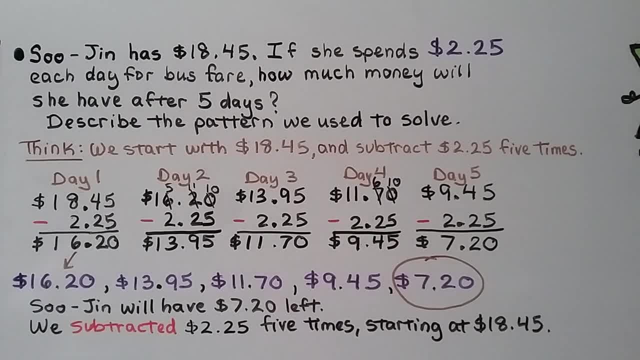 Describe the pattern we used to solve. So we think we start with $18.45 and subtract $2.25 5 times for the 5 days. We start with $18.45 and after subtracting her bus fare, we get $16.20. 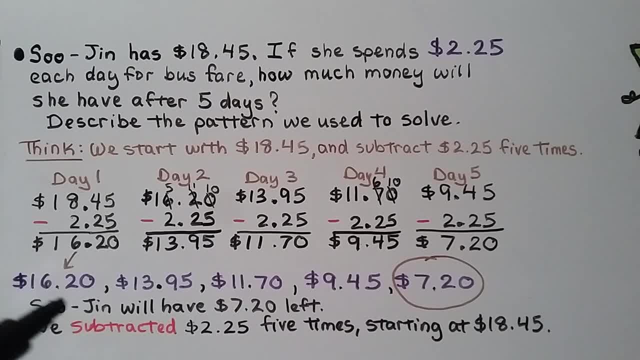 That's how much she has left. We subtract $2.25 from this amount to get our second term, and we subtract $2.25 from this amount to get our third term. We subtract $2.25 from this amount to get our next term. and for the fifth one, the fifth. 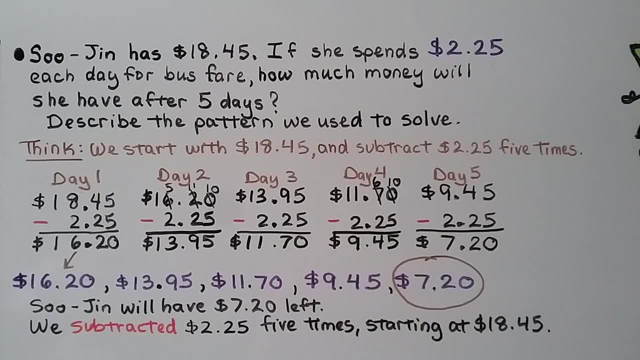 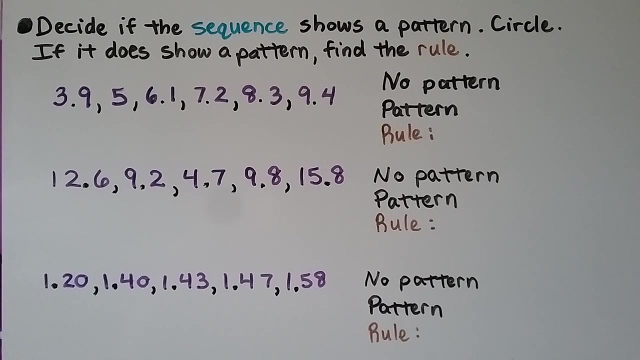 day we subtract it again and we see $7.20.. So Soojin will have $7.20 left. We subtracted $2.25 5 times, starting at $18.45.. It's telling us to decide if the sequence shows a pattern. 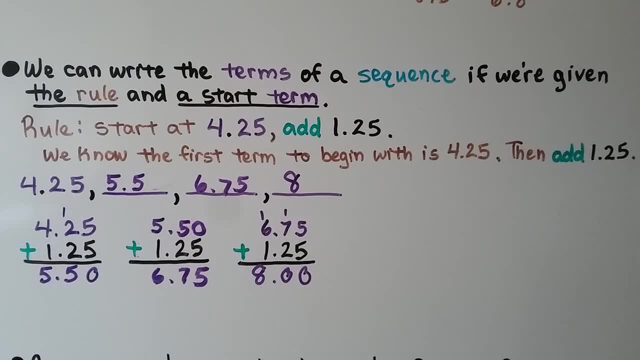 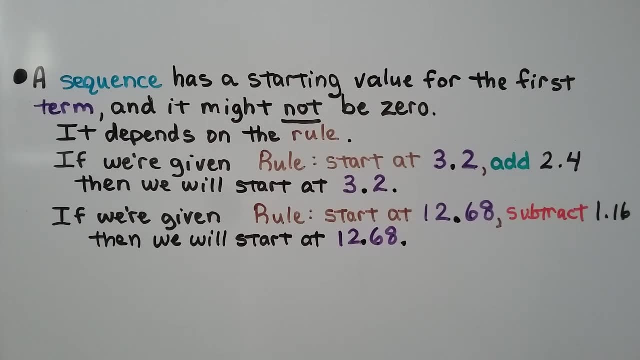 We can remove that trailing zero. A sequence has a starting value for the first term and it might not be zero. It depends on the rule. If we're given that the rule says: start at 3 and 2 tenths and add 2 and 4 tenths, 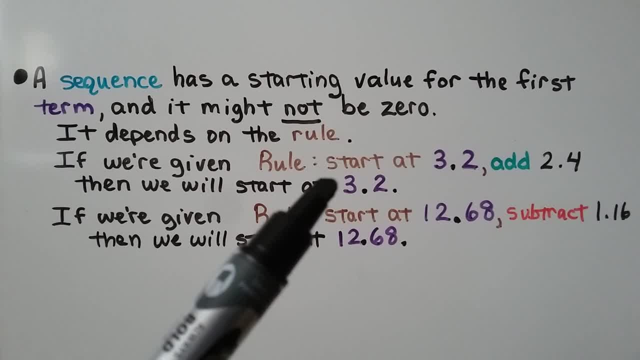 then our first term will be 3 and 2 tenths. That's where we'll start. Then we'll add 2 and 2 tenths, Then we'll add 2 and 4 tenths to it to get the next term. 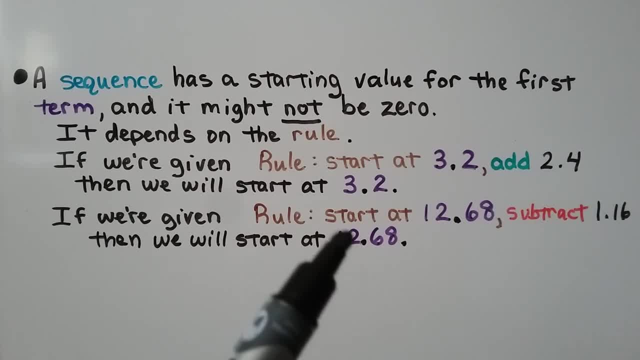 Add another 2 and 4 tenths And if we're given the rule start at 12 and 68 hundredths and subtract 1 and 16 hundredths, then we're going to start at 12 and 68 hundredths. 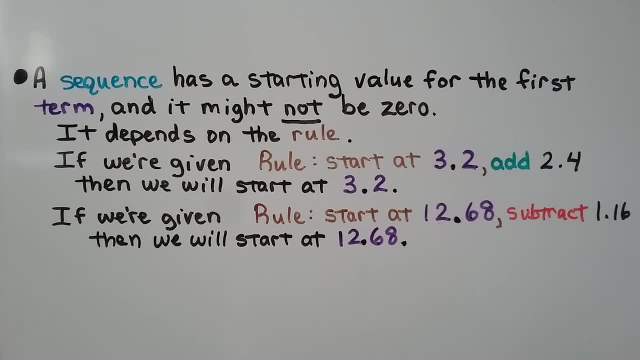 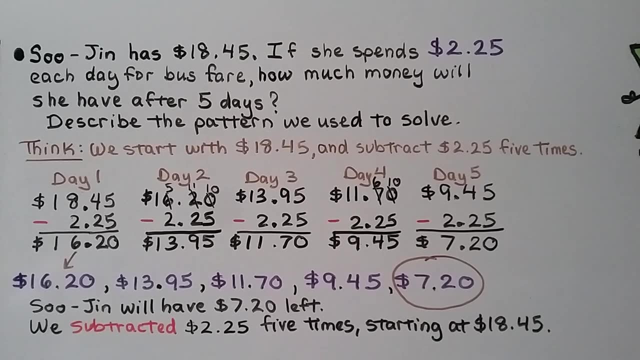 That will be our first term. Then we'll subtract 1 and 16 hundredths from it to get our second term. Soojin has $18.45.. If she spends $2.45, each day for bus fare, how much money will she have after 5 days? 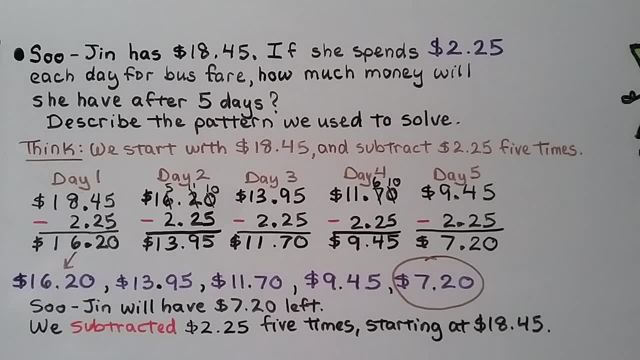 Describe the pattern we used to solve. So we think we start with $18.45 and subtract $2.25 5 times for the 5 days. We start with $18.45 and after subtracting her bus fare, we get $16.20. 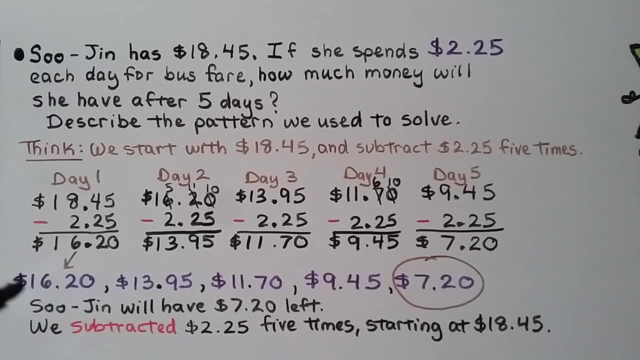 That's how much she has left on the first day. That's our first term. We subtract $2.25 from this amount to get our second term, And we subtract $2.25 from this amount to get our third term. We subtract $2.25 from this amount to get our next term. 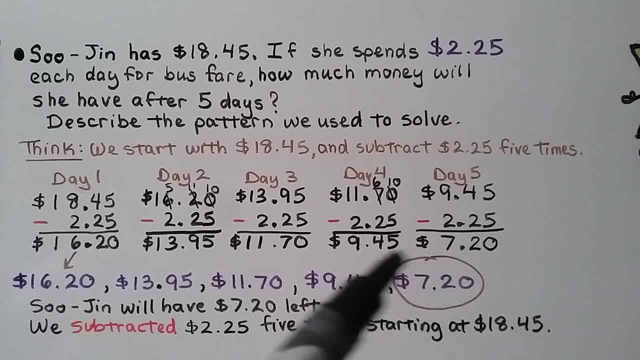 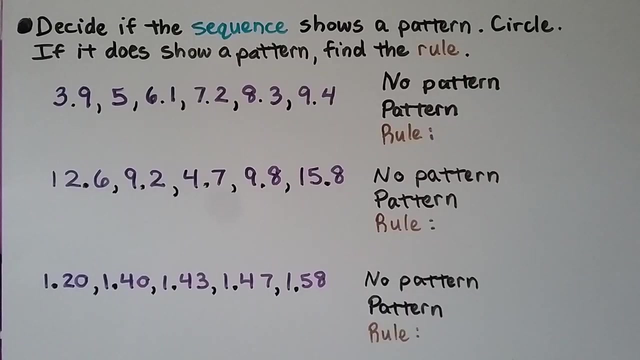 And for the fifth one, the fifth day, we subtract it again and we see $7.20.. So Soojin will have $7.20.. We subtracted $2.25 5 times, starting at $18.45.. It's telling us to decide if the sequence shows a pattern. 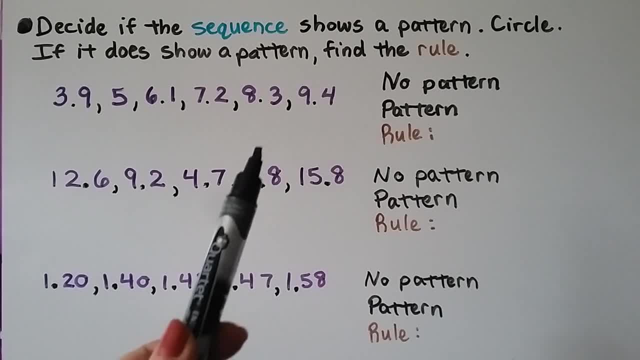 Then we need to circle no pattern or pattern And if it does show a pattern, we need to write the rule. We look at the digits and we see it's going from 3 and 9 tenths to 3 and 9 tenths. 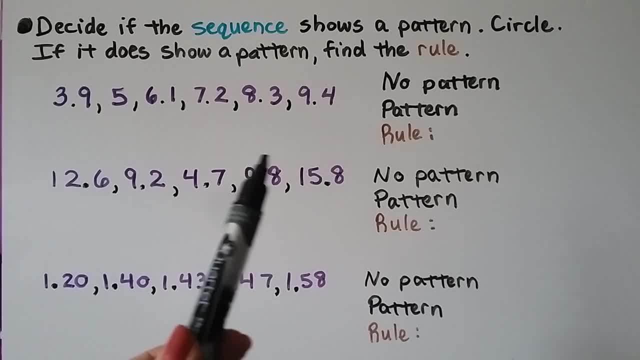 Then we need to circle no pattern or pattern and if it does show a pattern we need to write the rule. We look at the digits and we see it's going from 3 and 9 tenths to 5 to 6 and 1 tenths. 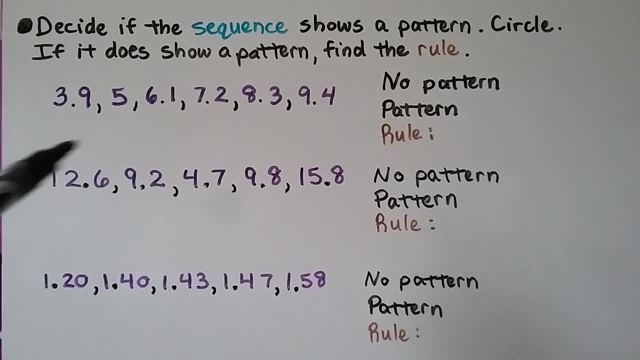 to 7 and 2 tenths to 8 and 3 tenths to 9 and 4 tenths. So it is increasing, So it's addition. So let's try subtraction to find the difference between 5 and 3 and 9 tenths, and then 6 and 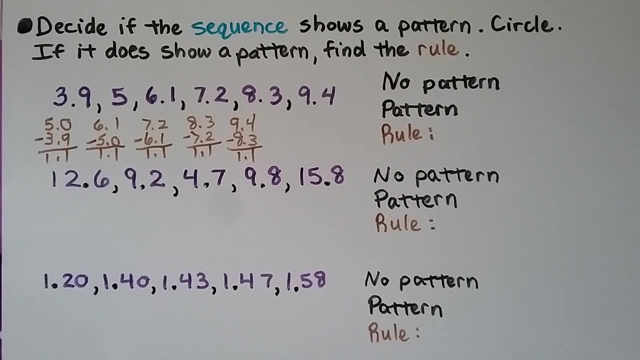 1 tenth and 5 and so on. We subtract, We look at each digit and find that they all have a difference of 1 and 1 tenth. So we know the rule is: add 1 and 1 tenth and there is a pattern because all of these have 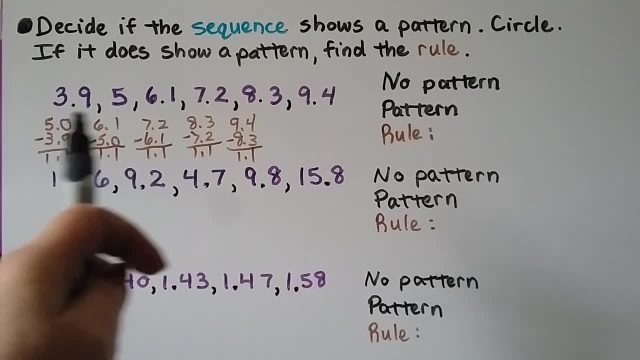 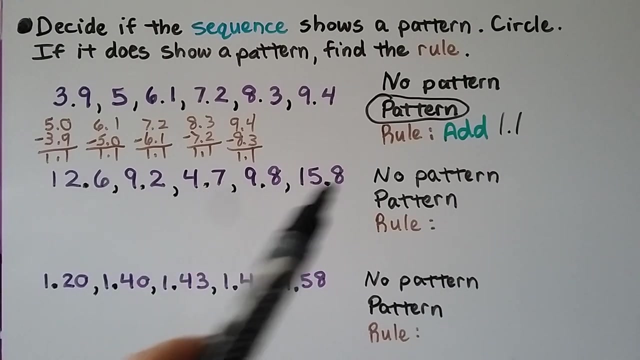 the same difference. The difference between each number is the same. So there's a pattern and the rule is to add 1 and 1 tenth. Now we need to compare the differences for these. We see 1 and 5 tenths in it's 9th and 6th, and it goes on backwards and down in it's 12th. 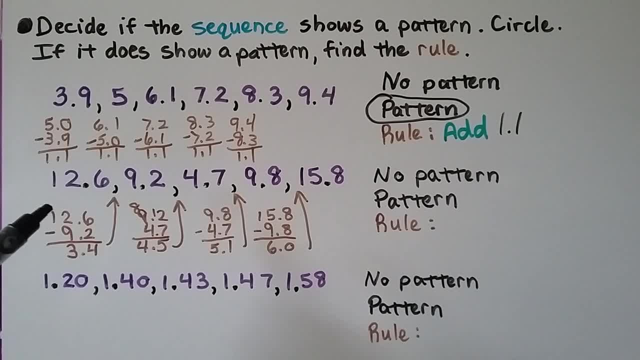 In subtraction. we use subtraction to find the difference between each number and we see that the 2 andberger strawberries have a difference in every way. We can see that in between 6 and 3 and 9 they all have the same meaning: 1 and 3 and 4.. 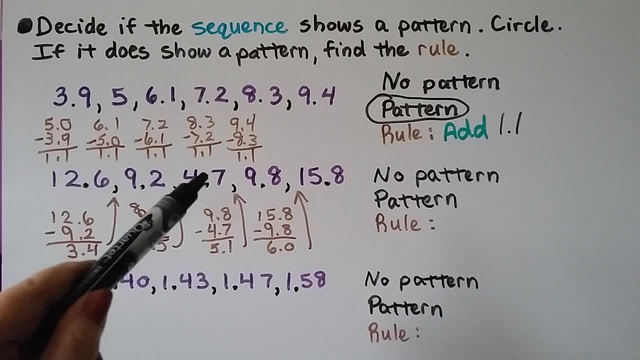 The difference between the 2 and 3 versions equals 4 and 5 tenths, and the difference between these two terms equals 5 and 1 tenth one-tenth, and the difference between these two terms is six. they're all different from each other, so there's no pattern for this one. we saw they all had. 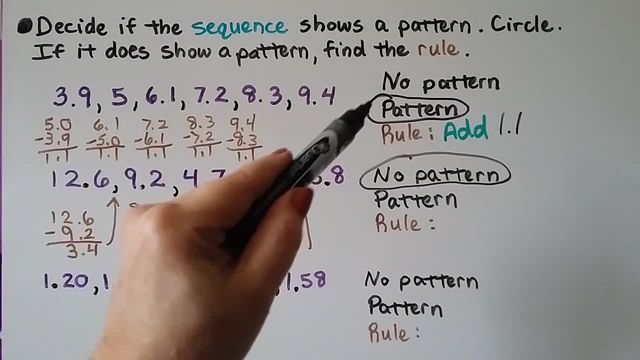 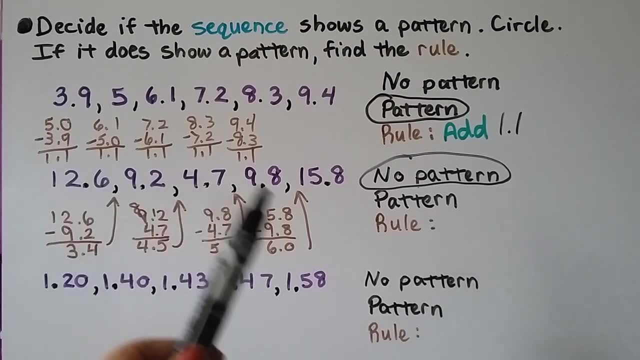 one and one-tenth difference between them. so there was a pattern and we knew the rule, because each of these have a difference that's different from the next set of terms. there's no pattern. let's try it with this one. we can see it's going from one and twenty hundredths to one and forty hundredths. 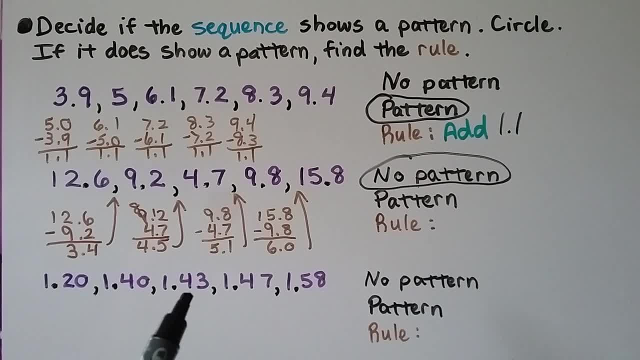 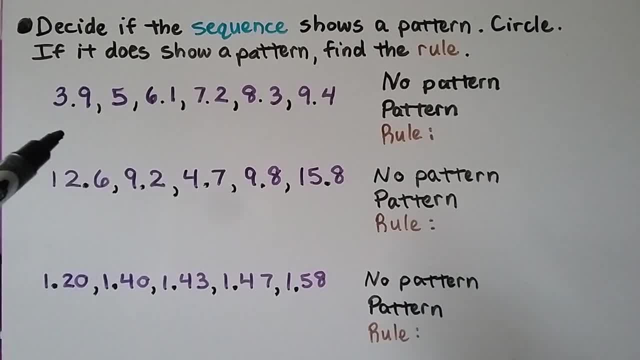 eight and three tenths to nine and four tenths. so it is increasing, so it's addition. so let's try subtraction to find the difference between five and three and nine tenths, and then six and one tenth and five and so on. we subtract each digit and find that they all have a difference of one and one tenth. so we 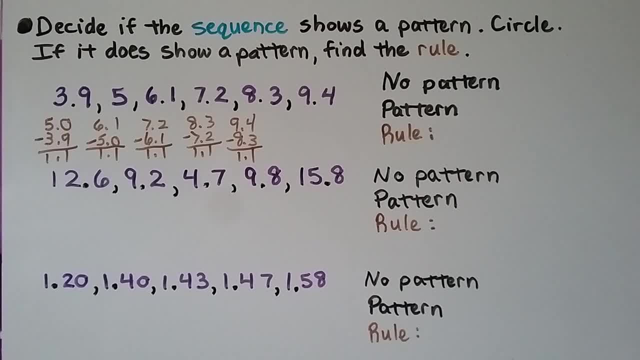 know, the rule is add one and one tenth and there is a pattern because all of these have the same difference. the difference between each number is the same, so there's a pattern and the rule is to add one and one tenth. now we need to compare the differences for these. we see it goes from 12 and 6 tenths down to 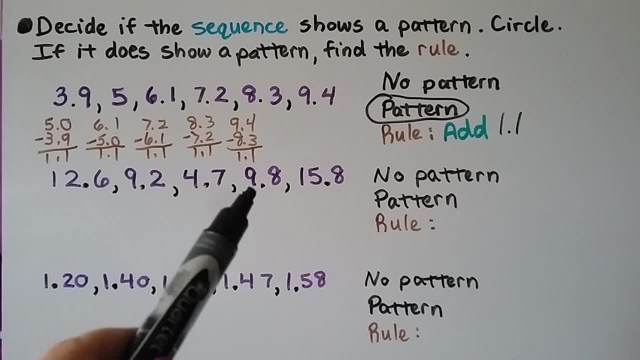 9 and 2 tenths, down to 4 and 7 tenths, but then it goes back up again and back up again. So let's find the difference between these terms. We use subtraction to find the difference between each term and we see that in between. 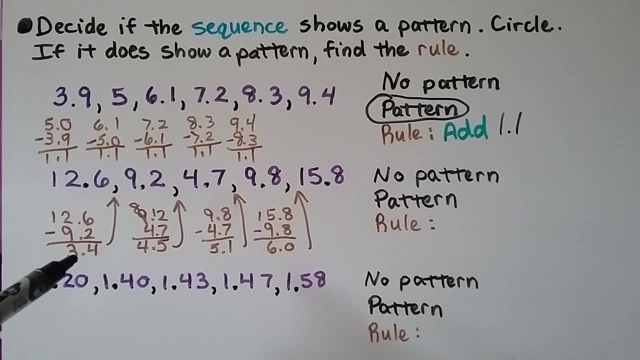 12 and 6 tenths and 9 and 2 tenths. we have a difference of 3 and 4 tenths, But the difference between these two terms is 4 and 5 tenths and the difference between these two terms is 5 and 1 tenth and the difference between these two terms is 6..